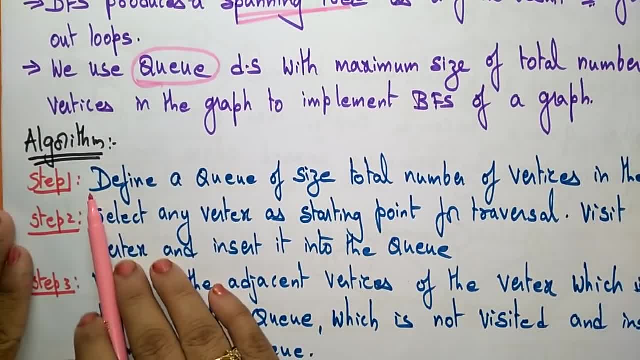 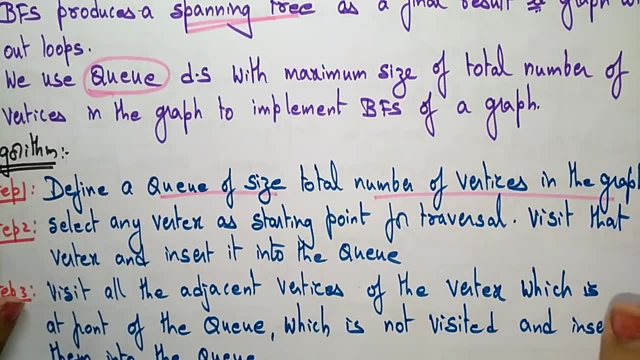 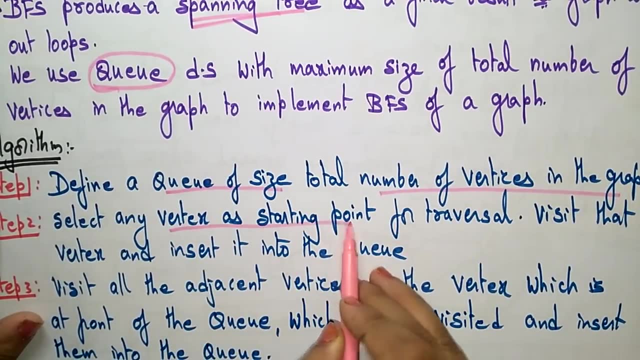 Based on this algorithm, we will implement the example. First define a queue size, So based on the number of vertices in the graph. so how many vertices are present in the graph? based on the vertices, you just first define the size of the queue, Select any of the vertex as a starting point. So, just like DFS, just select any of the vertex for traversal, visit that vertex and insert into the queue. So first element was inserted in the queue. So queue means first in, first out. Whatever the element, first you insert. 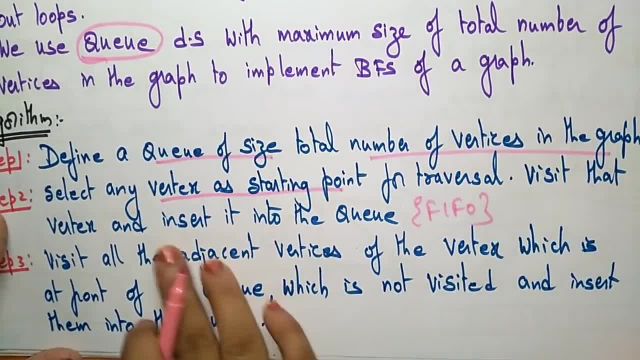 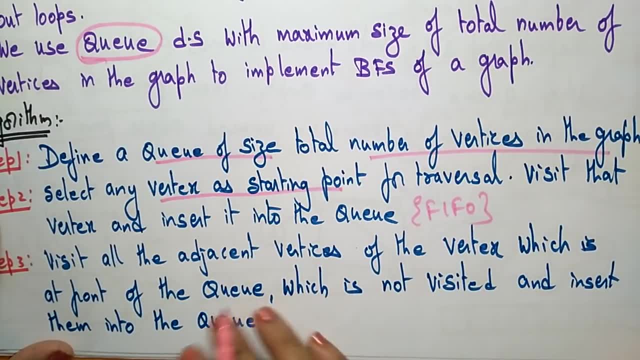 inserted that should be out from the queue. visit all adjacent vertices of the vertex which is at front of the queue which is not visited, and insert them into the queue. so here what i was saying, whereas in dfs you have to visit one of the vertex which is adjacent to that vertex. 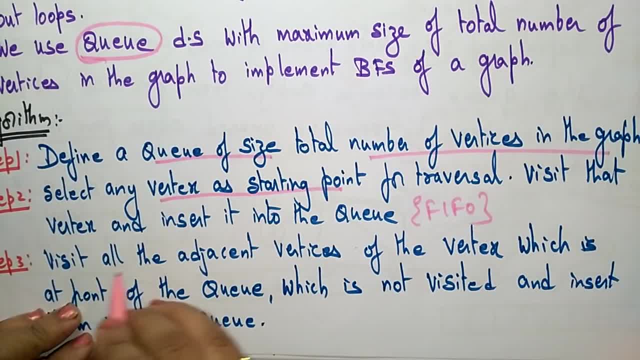 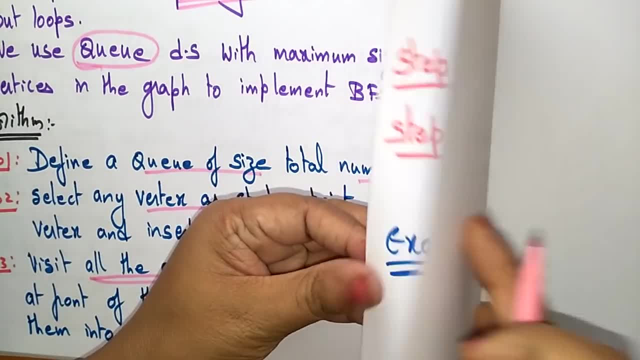 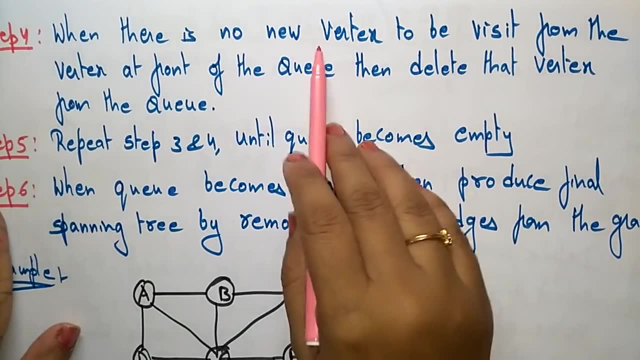 so just take one of the vertex, but here in the queue you have to visit all the adjacent vertex and you have to place in front of the queue. so next step four, when there is no new vertex, let us take, if you, you enter all the vertices when there is no new vertex to be visit from. 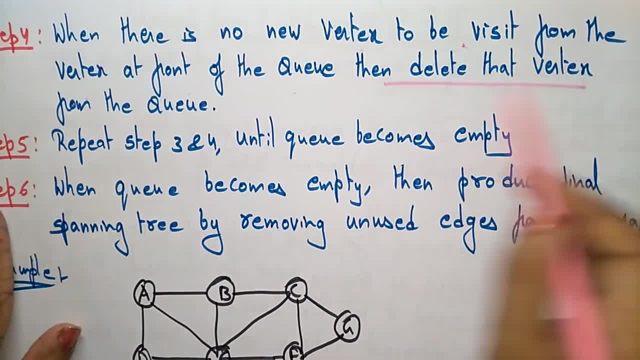 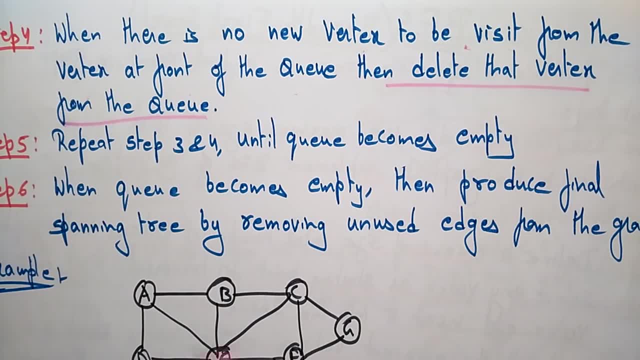 the vertex at front of the queue, then delete that vertex from the queue. so when there is no elements vertex that you have to be placed on the queue, just delete the element. that is the first in fast out element. in the way, just repeat the step three, four until the queue becomes. 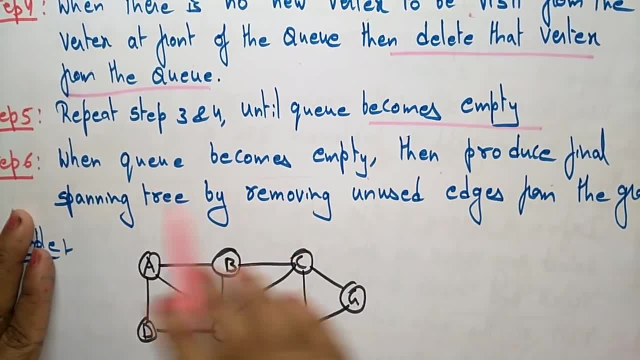 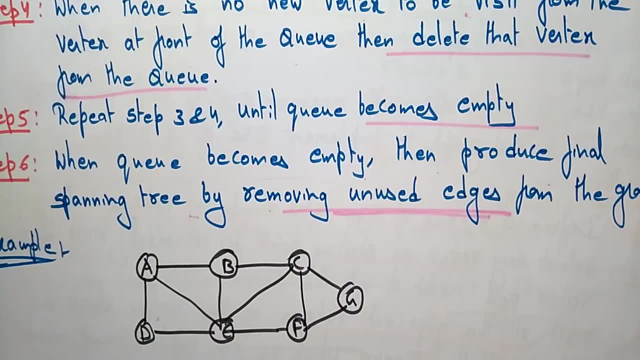 end empty. so whenever the queue becomes empty, then produce a final spanning tree by just removing the unused edges. so whatever the unused edges that are present in the graph that should be removed. so here i am taking the same example, whatever i have taken for the dfs, so that you 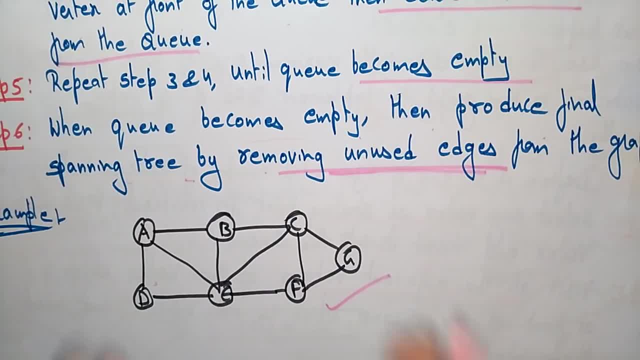 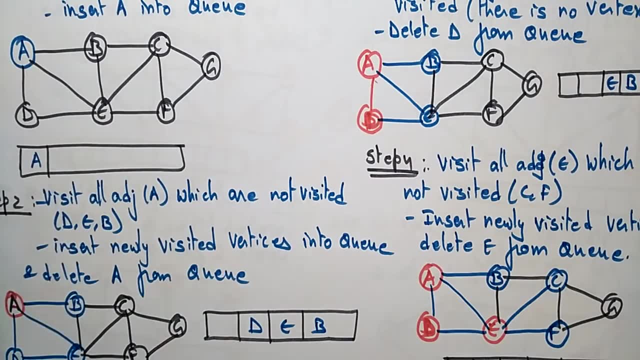 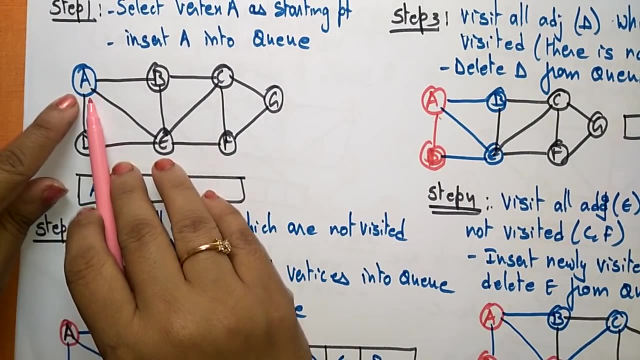 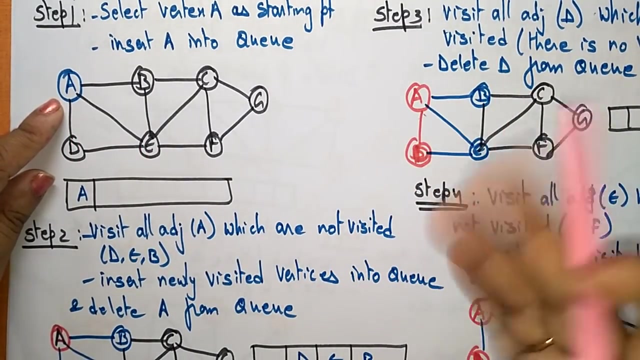 will compare the structure of the graph, how the same graph will be represented in dfs and bfs. so let me explain with example. so select first whatever the graph i am taking. so just select vertex a as a starting point. so here i'm marking as a blue indicates the visited vertex and the black is or unvisited vertex and red or the deleted from the. 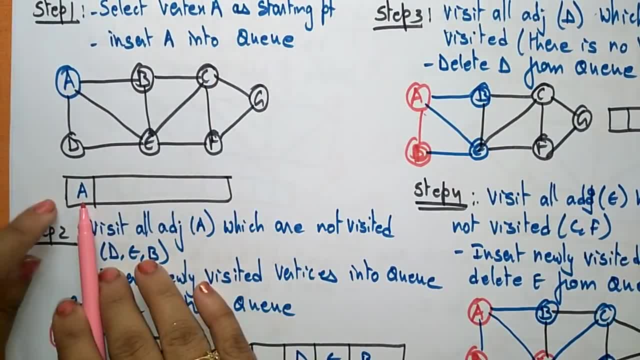 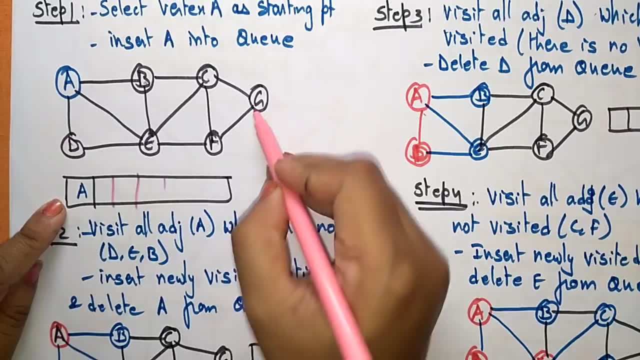 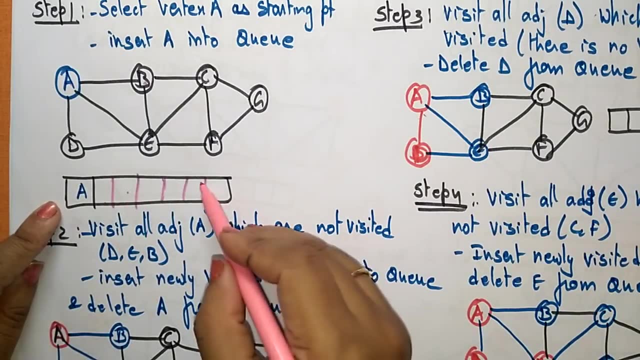 queue. so select a as a starting point and placed it on the queue. so the queue size. what is the size of the queue? number of elements: 1, 2, 3, 4, 5, 6, 7. so 1, 2, 3, 4, 5, 6, 7. okay, total the size of the queue is: 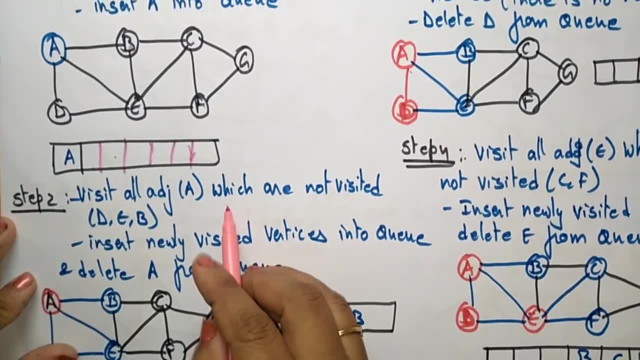 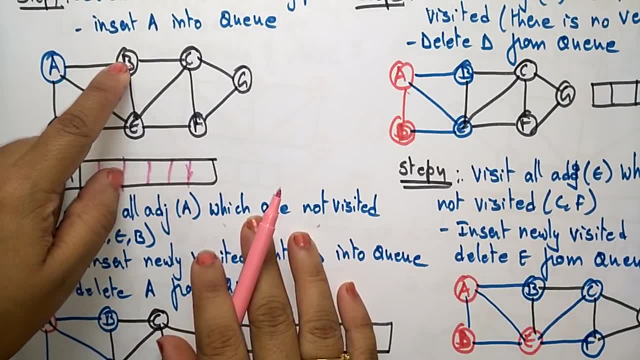 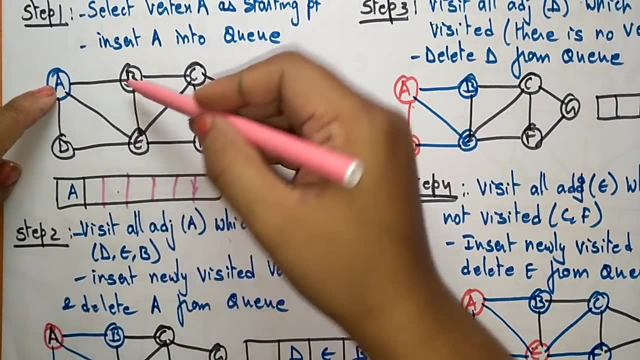 7. So visit all adjacents of A which are not visited. So just in the DFS you are just placing whatever the adjacent vertex. you are just taking one of the vertex adjacent vertex, but in the BFS, so in the Q, you have to just select all the adjacent vertex of the A. What are the adjacent? 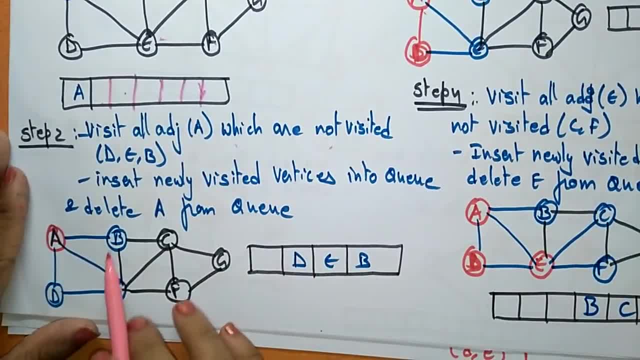 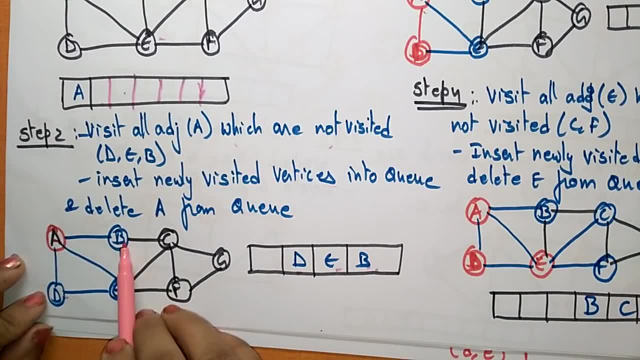 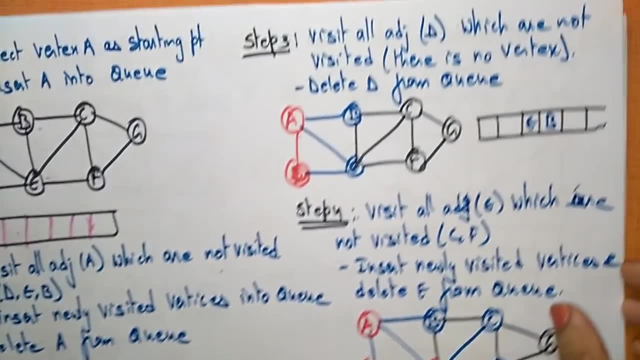 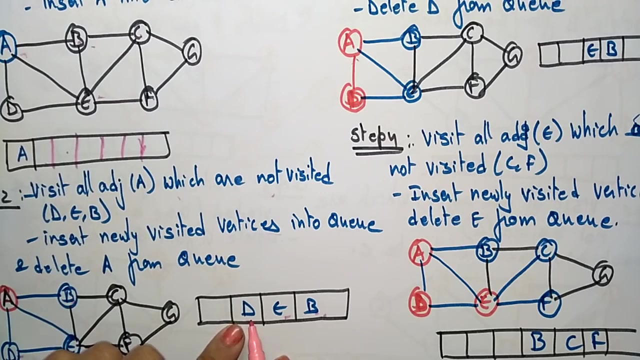 vertex of A, D, E, F. So just insert newly. insert visited vertex in the Q, D, E, D, E, B and just delete A. So whenever you are inserting the adjacent vertex, just delete A according to the algorithm. Next visit all adjacent of D. So now I am taking this is the first in is D, So 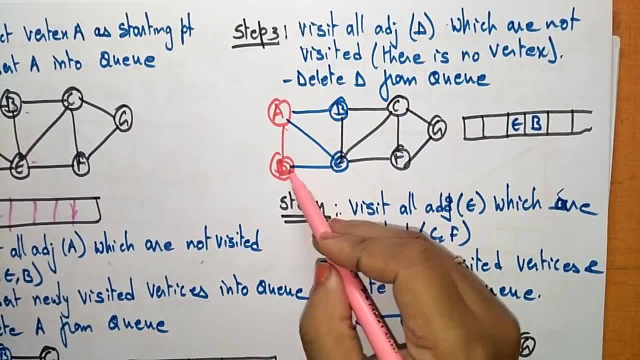 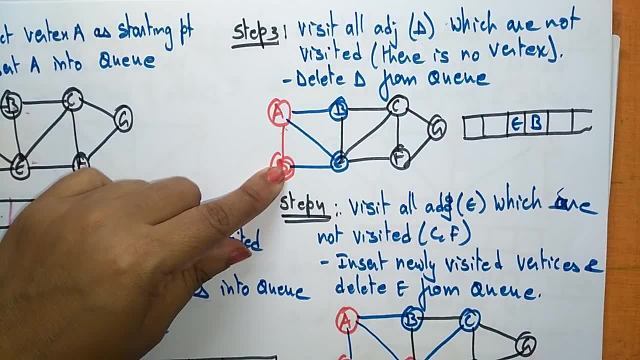 visit all adjacent of D, which are not visited. So from d there is only a and e are there, but they are already visited. so according to algorithm, if already visited vertex are there. so just delete the d from the q. so i deleted d from the q. 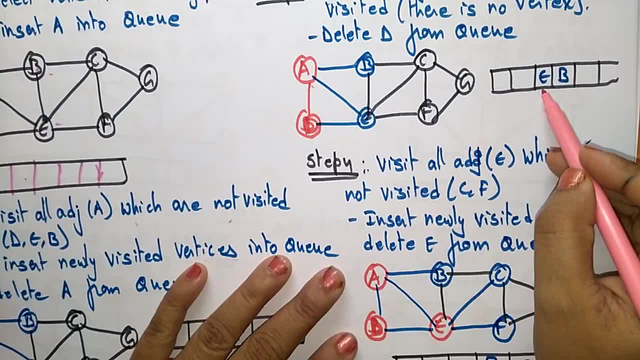 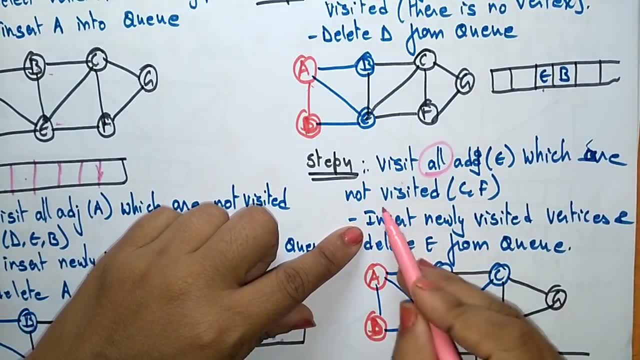 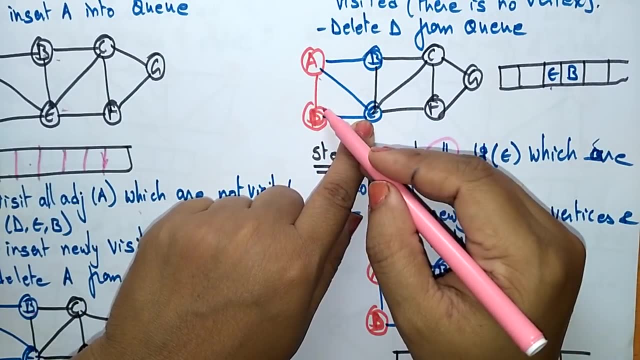 now e. e is the adjacent vertex we have to check: visit all edges. so you have to remember this: all visit all edges which are not visited. so from e, what are the non-visited edges? so b is visited, d is visited, a is visited, c, f are not visited. so just insert into the q. 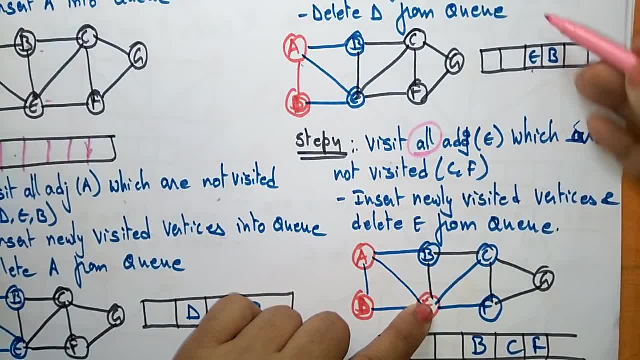 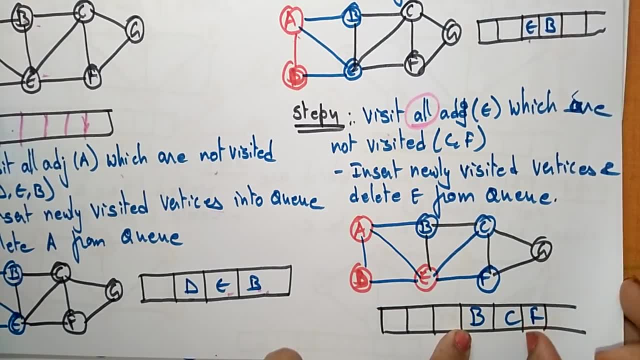 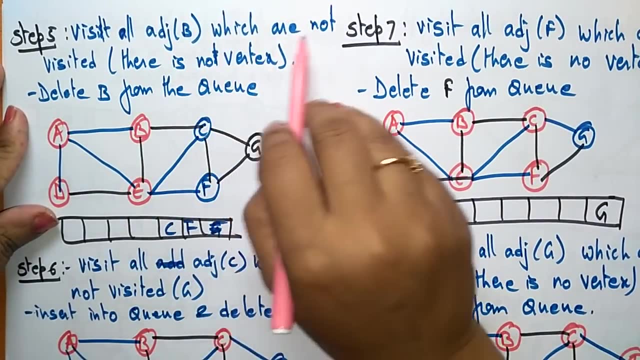 and delete e. so whenever you insert into the q you have to delete that from the q. so after b you have to place c, f, now b you have to check the b. so b is the adjacent vertex now visit all adjacent of b which are not visited. so from b which are: 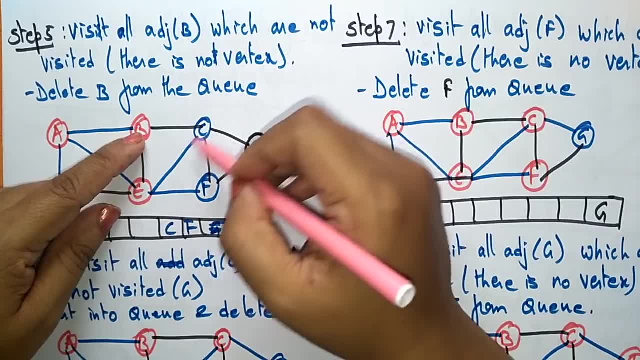 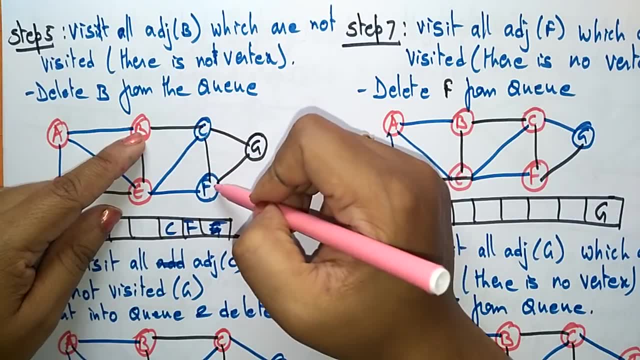 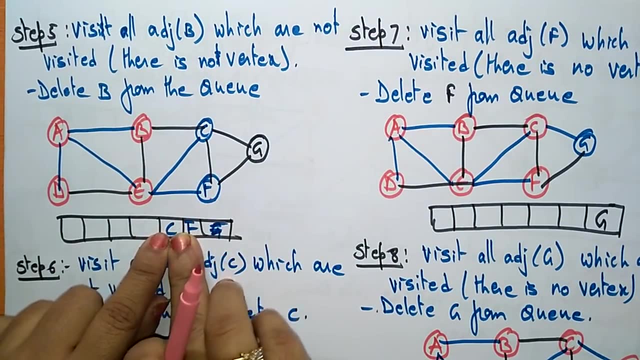 not visited. okay, c f is already visited. okay, the blue lines is already, blue circles is already visited. c f is already visited. so there are no vertex to be visited. so just delete b from the q now. next adjacent is c. you have to be checked. visit all adjacents of c. now i'm checking the adjacents.